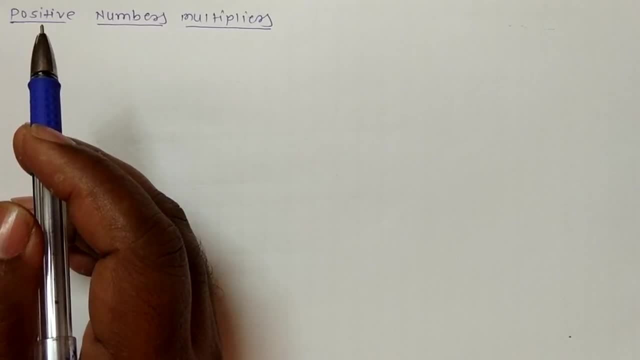 unsigned numbers, that is, positive numbers, Okay, and then we will see the multiplication algorithms for signed numbers. Okay, in this lecture only we will see what the multiplication of unsigned numbers, that numbers, means what positive numbers, Okay, so we take one example and we'll see how that multiplication is done in using or in binary form, right? So here example. 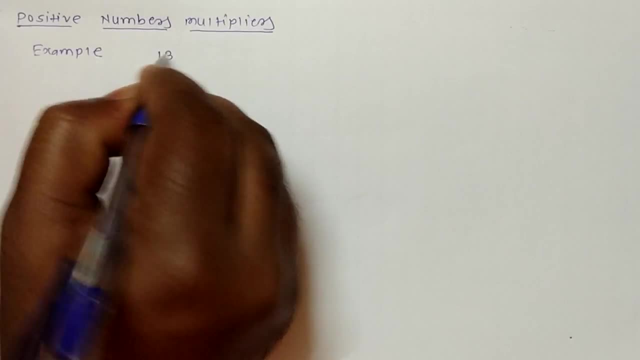 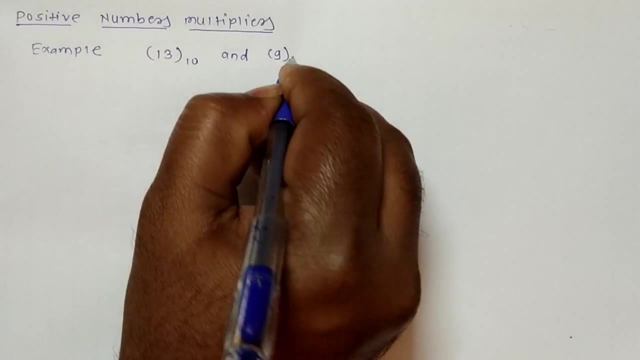 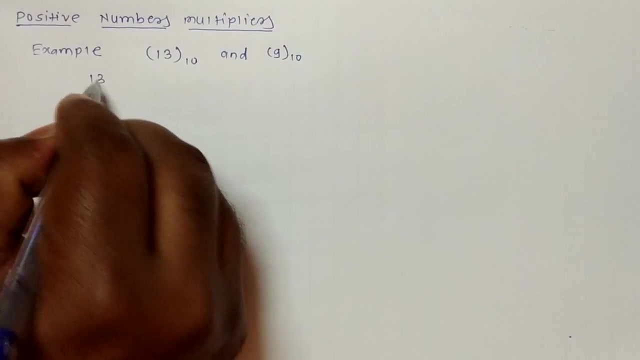 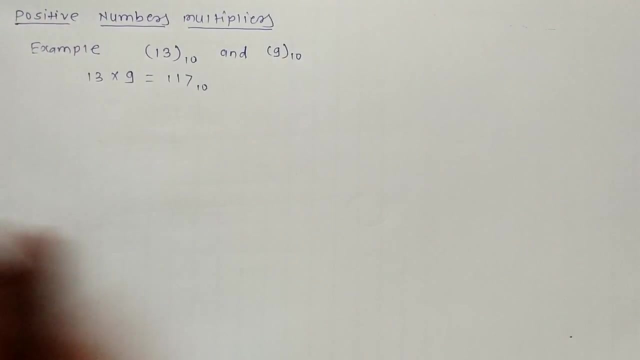 for it right. Suppose we have to multiply 13,, which is in decimal, and nine right. Take any example, right? So here we are. we are taking all 13 and 19.. We know 13 into nine. what will be the result? 117 in decimal right. So convert these numbers in binary, So 13,, which is in decimal. 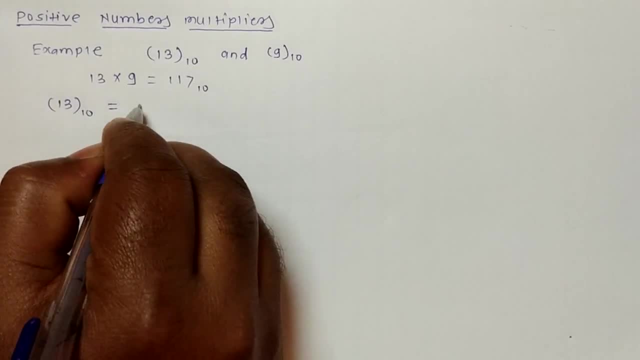 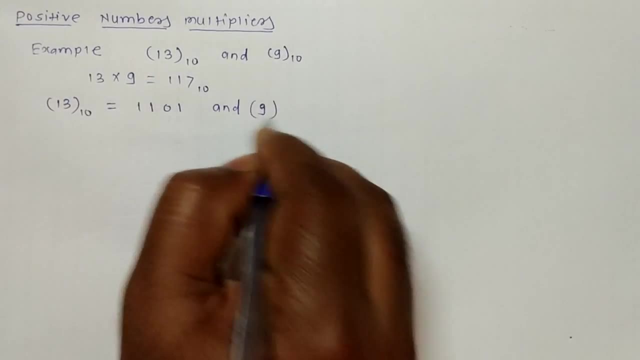 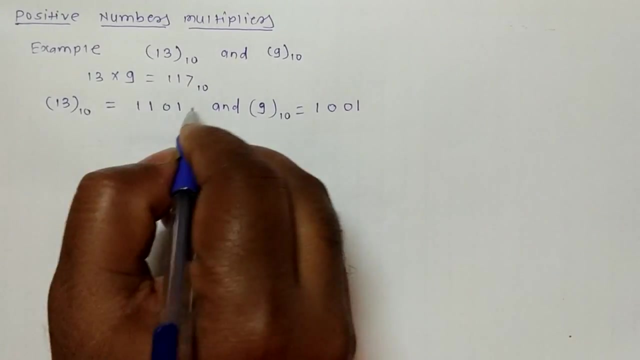 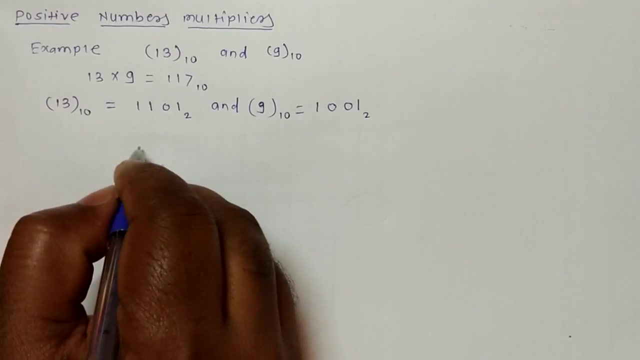 have to convert in binary. so what? what is the value of it? one one, zero one and nine is what 19 decimal is equal is equal to one zero, zero one, which is in binary. i'll write here: two means one binary. okay, so we have to multiply these two numbers. so i'll multiply this so one. 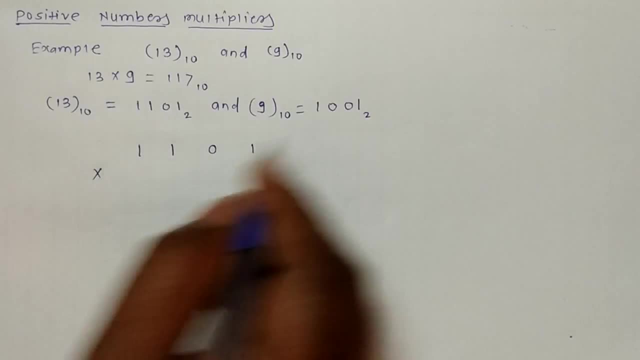 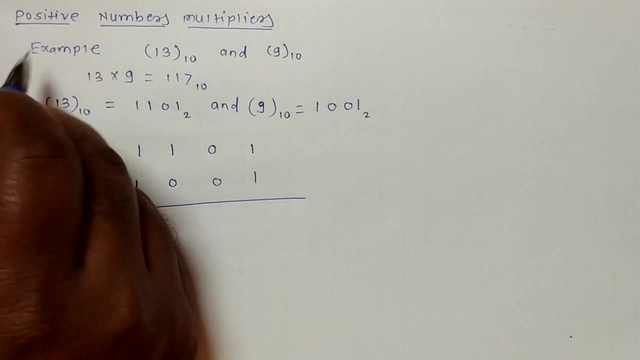 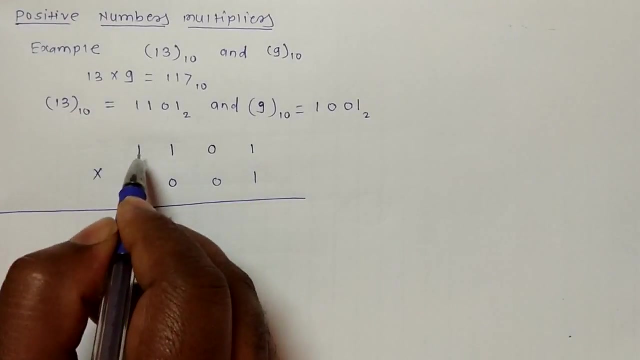 1 0 1 into 1 0 0, 1. remember, these numbers are positive numbers. we have to perform what positive numbers multiplication. so we, these two numbers are positive numbers, even though year one is there. but these are what positive numbers we can append. 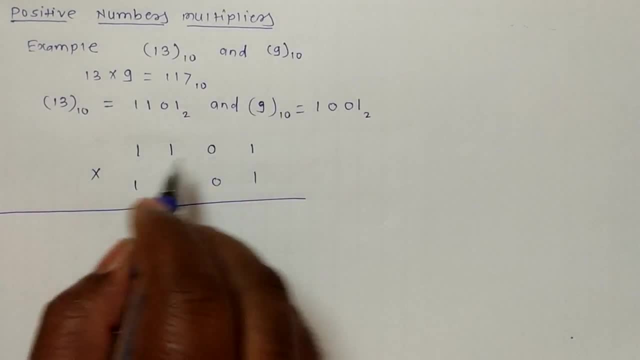 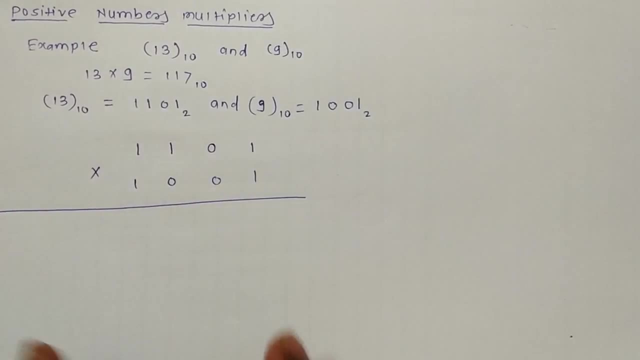 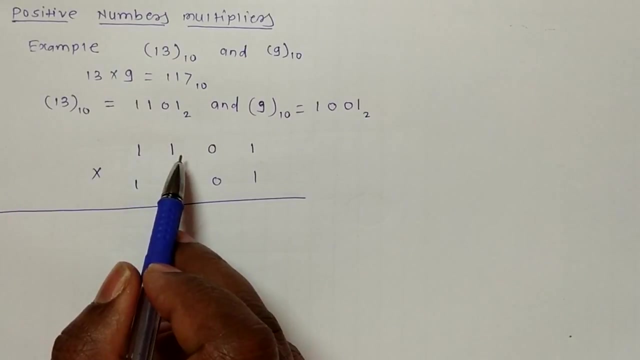 here: 0, no problem, okay. so remember these are what four bit numbers and the multiplication after performing the multiplication. multiplication, whatever the result we are getting, that result will be of 2n. any four bits are there, so we will get what eight bits result. so when you are performing the addition- uh, sorry, multiplication. 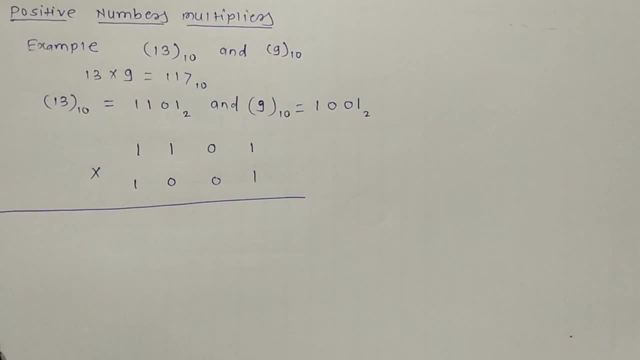 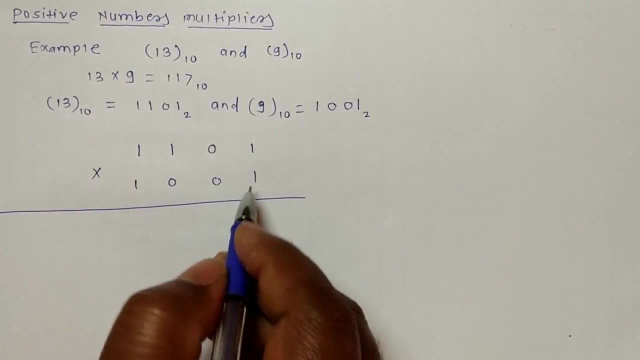 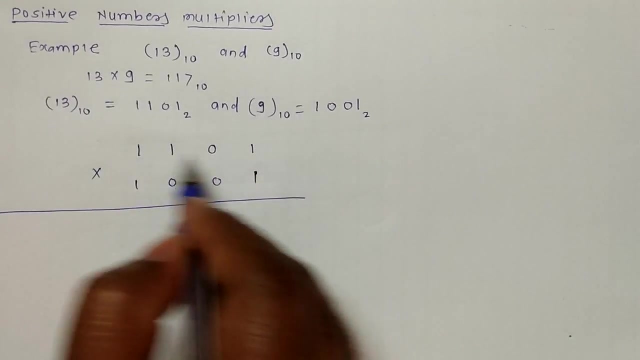 of n bits, then you will get what the result will be of 2n bit. okay, so see if i have to find what the partial product from it, and then we have to add the partial products. okay, so if we are multiplying by one, then you have to write multiplicand. this is what the multiplicand right.